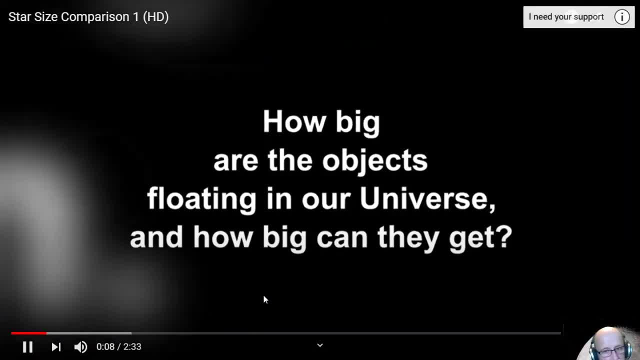 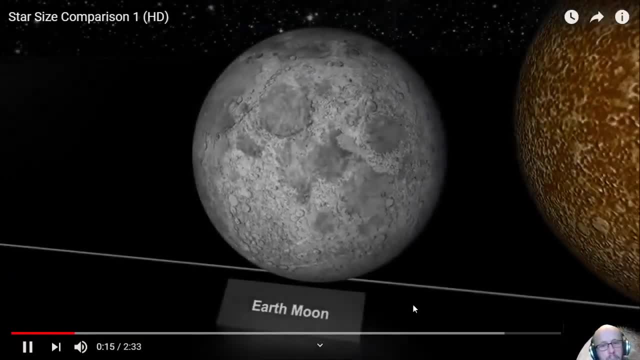 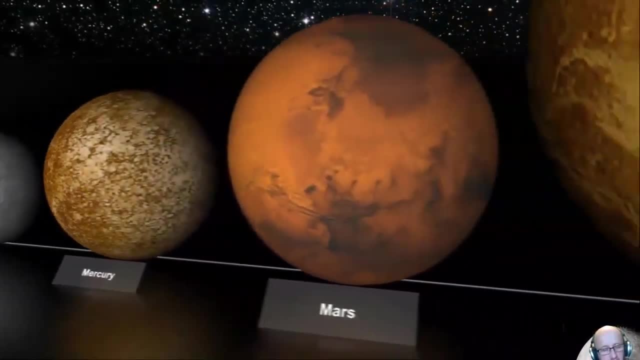 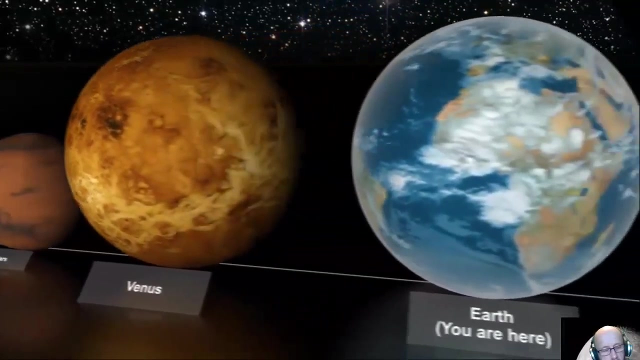 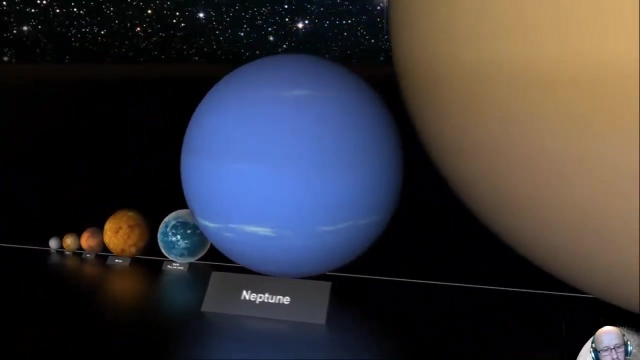 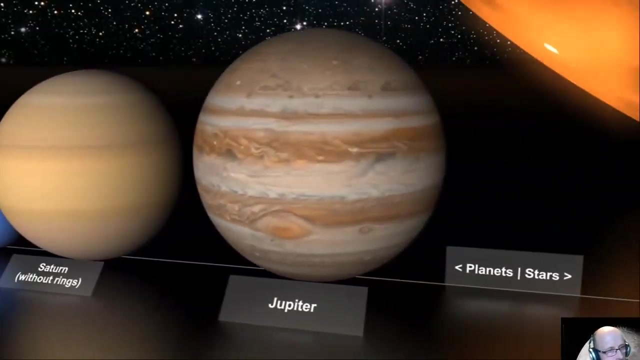 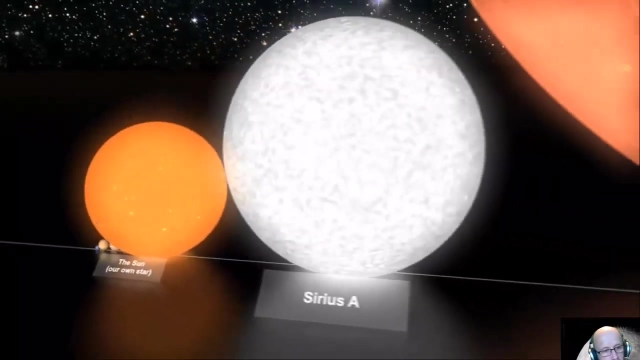 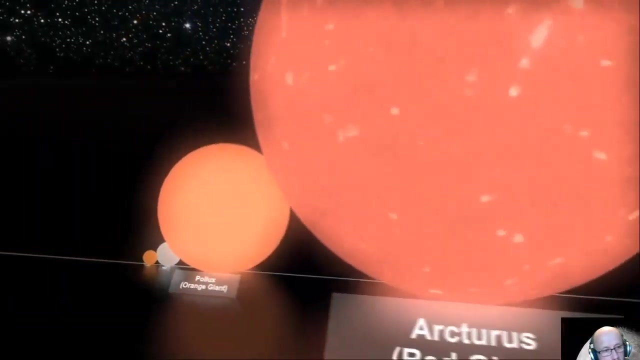 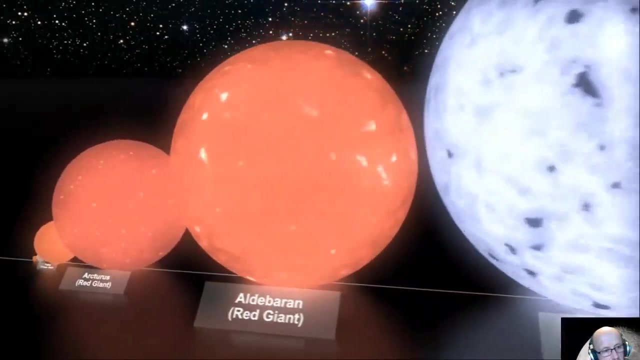 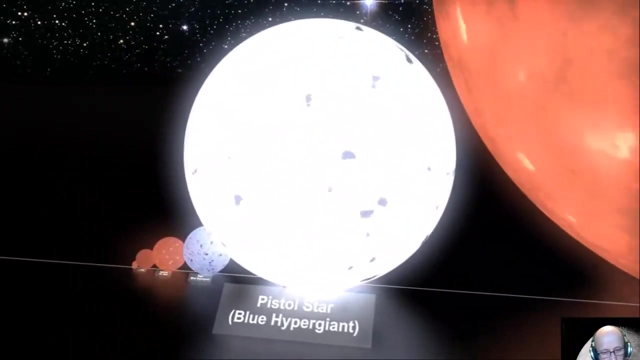 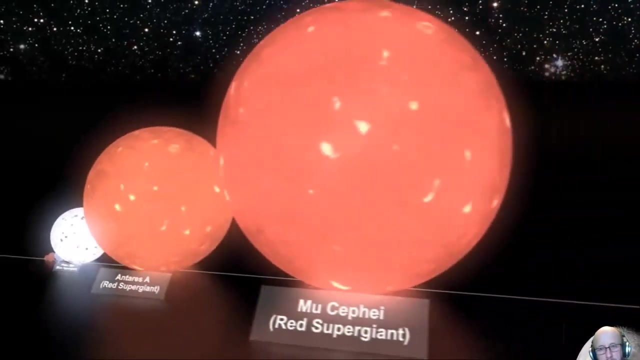 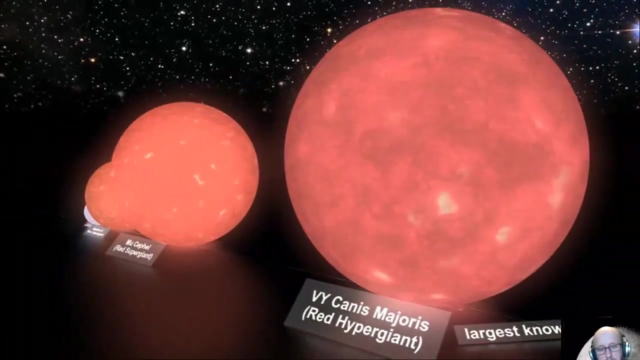 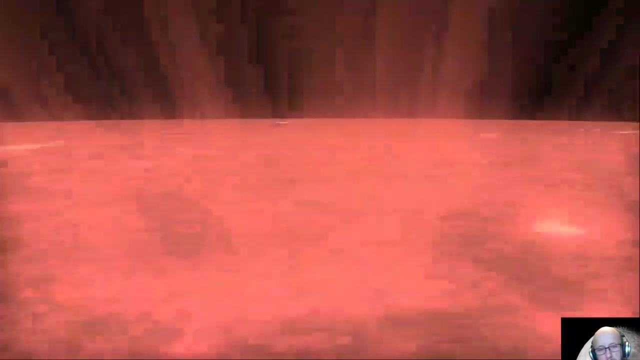 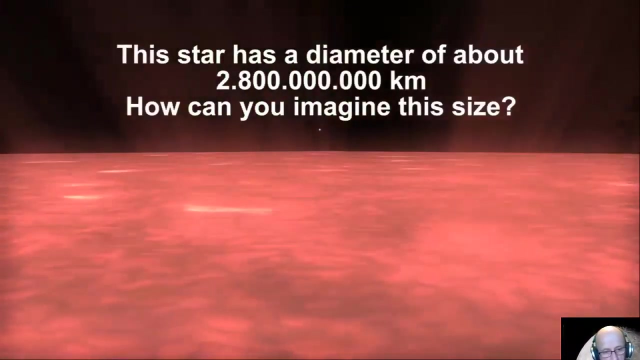 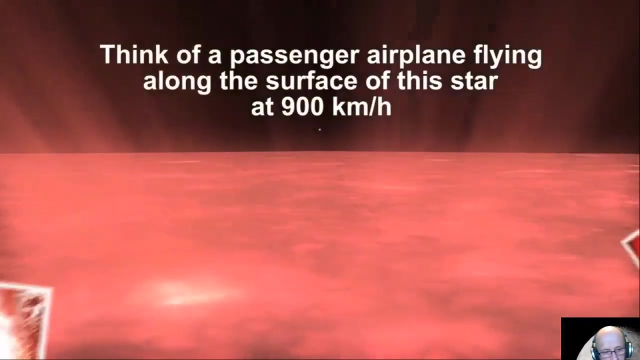 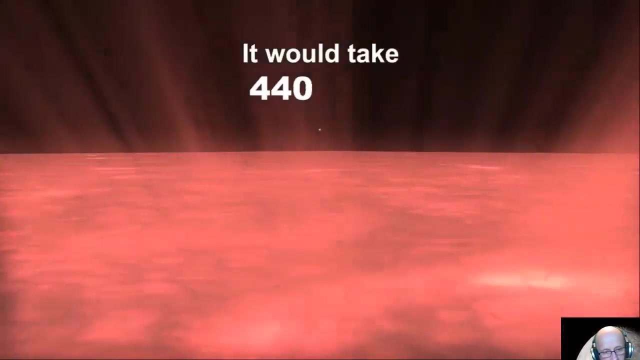 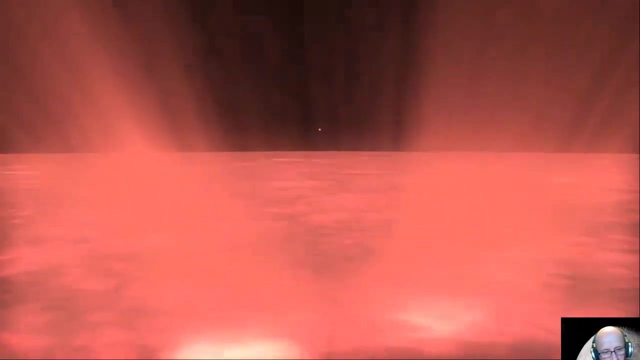 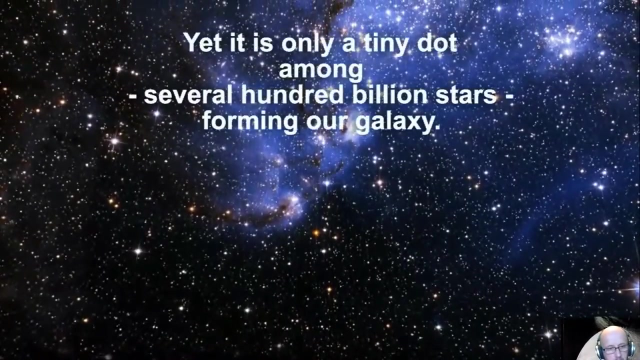 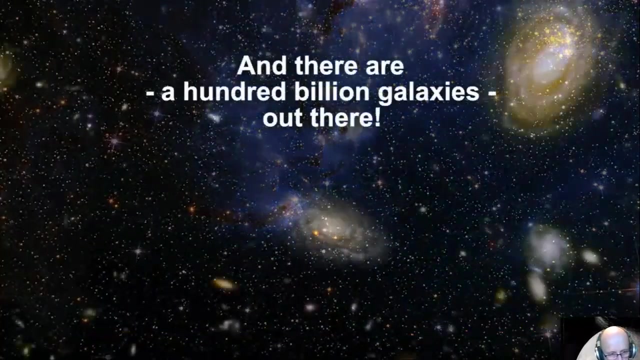 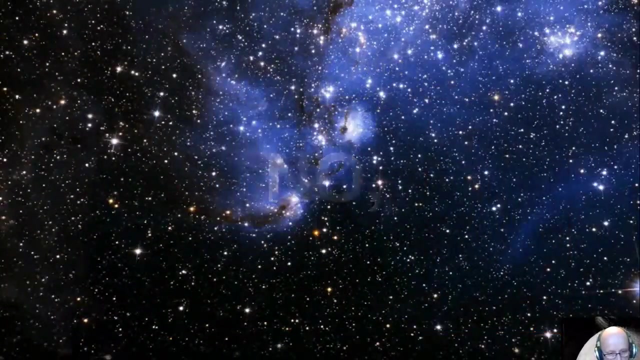 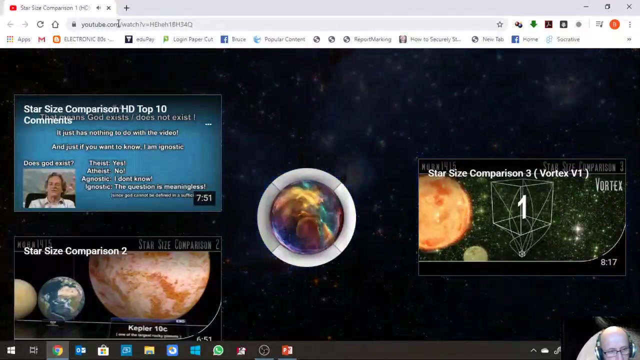 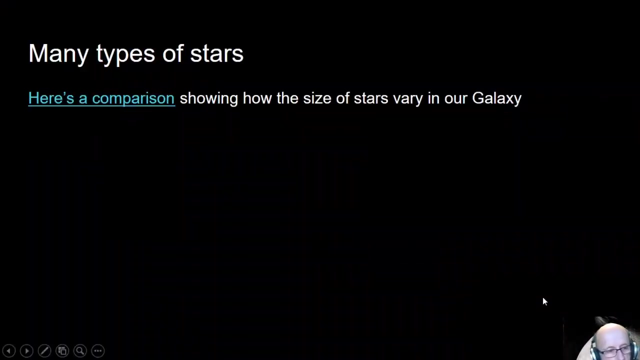 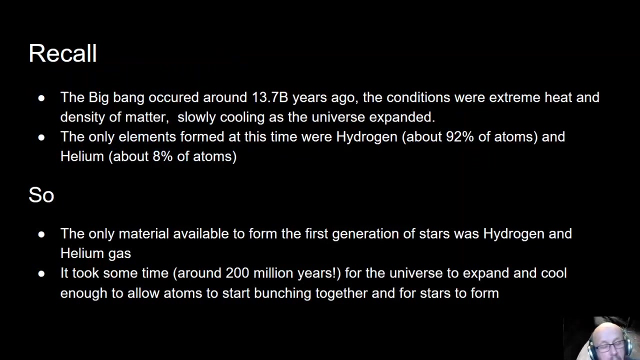 So so, so, so, so, Okay. so so from the video that we just watched you can see that there is a wide variety of star sizes and colors. So hopefully from the first powerpoint you can recall that there's a lot of evidence that there was a big bang that started 13.7 billion years ago, and some of the evidence 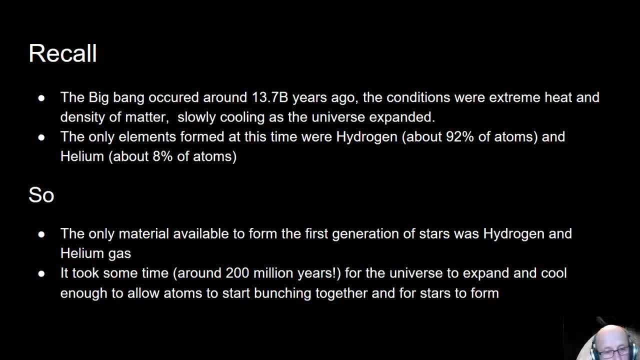 includes the type of elements that we have, which is hydrogen helium, the lightest elements- they're 92% of all atoms- but also the remnant of the big bang's energy, which is seen in cosmic background, microwave radiation, which you see all around the universe and indicates the heat. 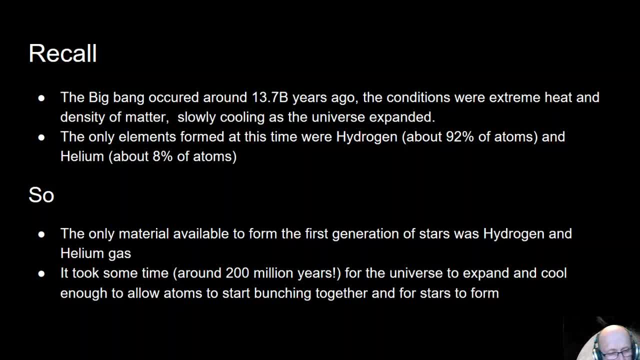 of the big bang. So the only material that is available in the first generation of stars is basically hydrogen helium- the lightest atoms, and it took about 200 million years for the universe to cool enough so that atoms could start getting close enough together for stars to form. 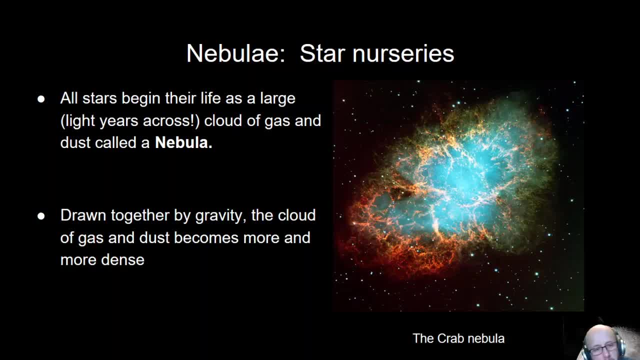 Now, if you look around space, you will see clouds in the sky to the naked eye. You can see them. Those are called nebulas and they are star nurseries. Basically, nebulas are where stars begin their life. they're are clouds out in outer space and they are light years across. 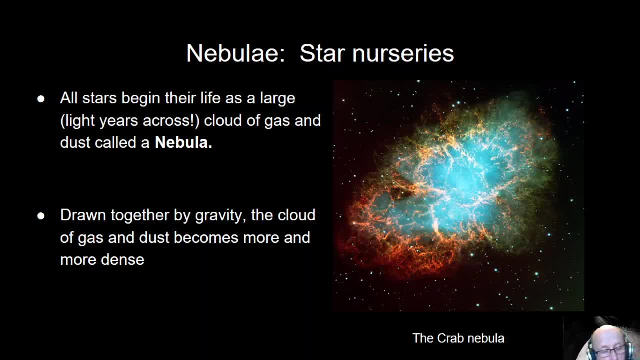 they are made up of dust, primarily hydrogen and helium, and we call these a nebula. They are drawn together by gravity and these become more and more dense because gravity is pulling them in. Now, some of the most famous nebula nebulas are the crab nebula, orion's. 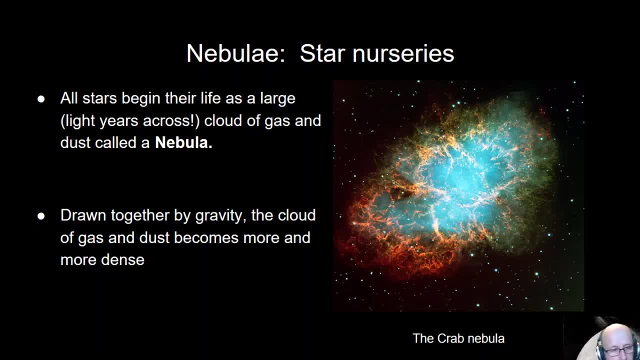 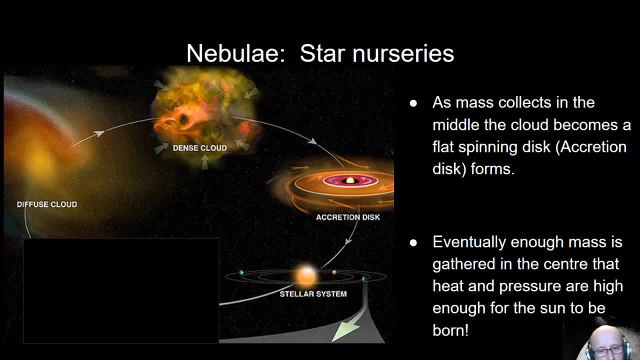 nebula and the Horsehead nebula. Nebulas are basically star nurseries. As mass collects in the middle of the cloud, it becomes a very flat spinning disk and it is very flat like an accretion disk, it's called, and it looks like a saucer. Now what is actually happening? is that the matter? 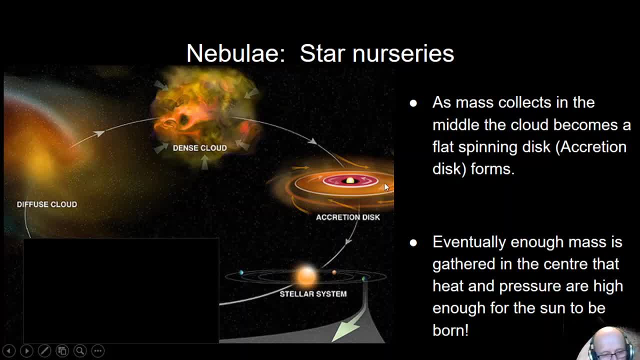 that is spinning around is being held up by angular momentum and being drawn in by gravity, and it holds it in balance, and that's pretty much what happens with our solar system as well. Those things above and below aren't spinning around, and so they either escape, if they're 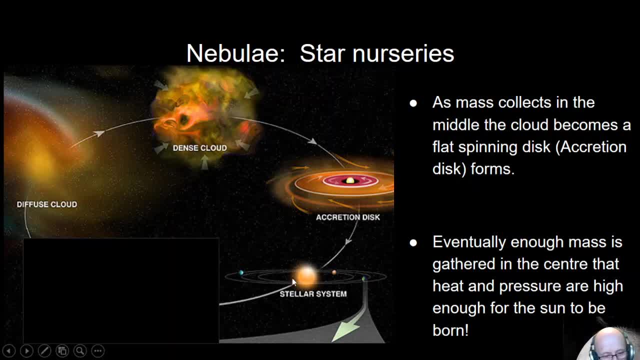 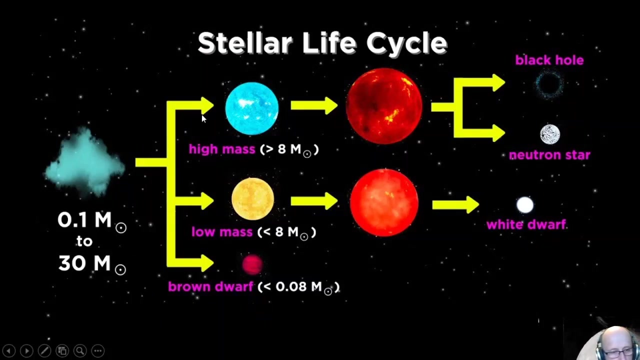 moving outwards, or they're drawn in by gravity. So basically, solar systems become flat disks And eventually they get enough mass in the middle that heat and pressure are high enough for a sun to be born. Now, overall, you will need to memorize this, this powerpoint. 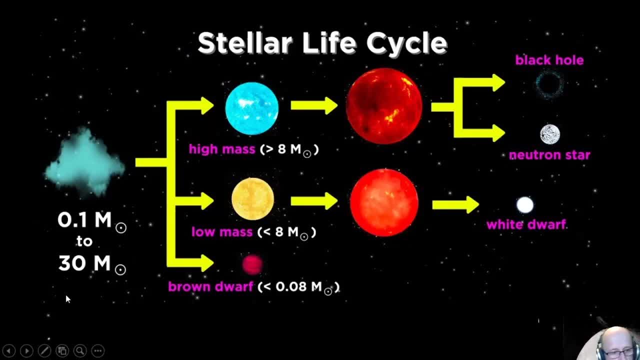 This is the different types of life cycles, but I just want to point out a couple of similarities. Whatever the size of the, the star turns up red and depending upon the mass of the star, it will have a different outcome eventually. So we've got brown dwarfs. they're smaller than our sun. 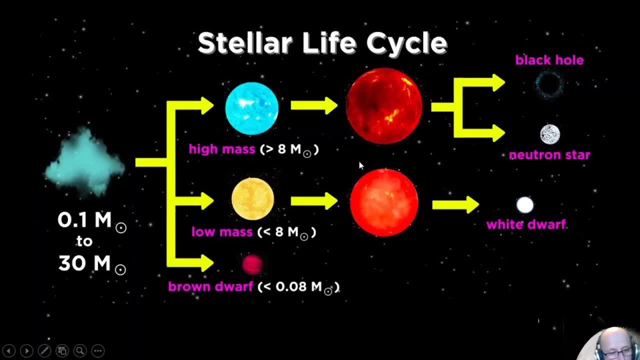 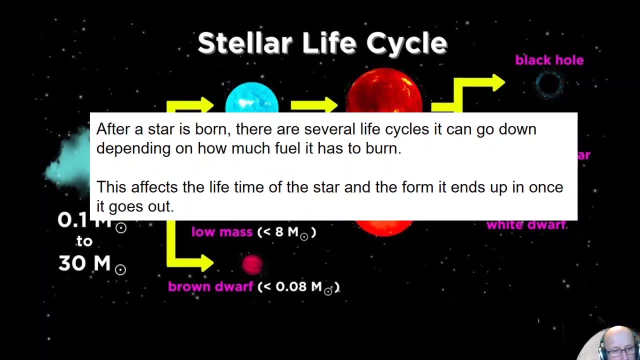 We've got low mass stars, like our sun, and we've got high mass stars. After a star is born, they can all those different pathways depending upon its mass. Now, a star doesn't actually burn. It's not like combustion. It releases energy via. 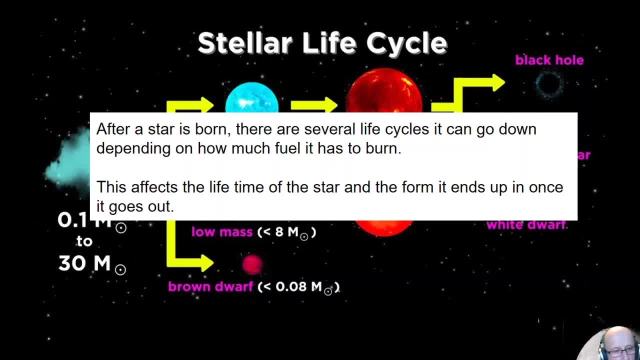 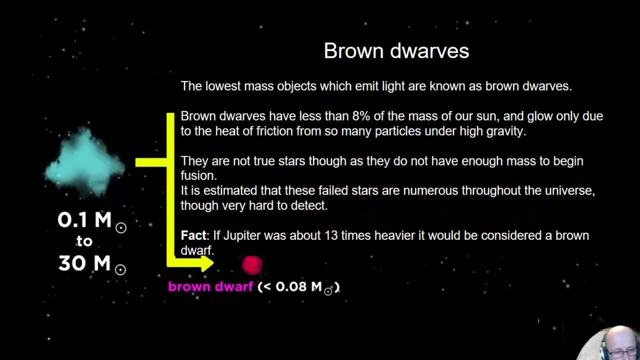 nuclear fusion. This affects the lifetime of the star and the form it ends up in once it goes out. Now the lowest mass star is known as brown dwarfs. Now, brown dwarfs are smaller than our sun. They're about 88% of the mass of our sun and glow only during due to the friction of so many particles. 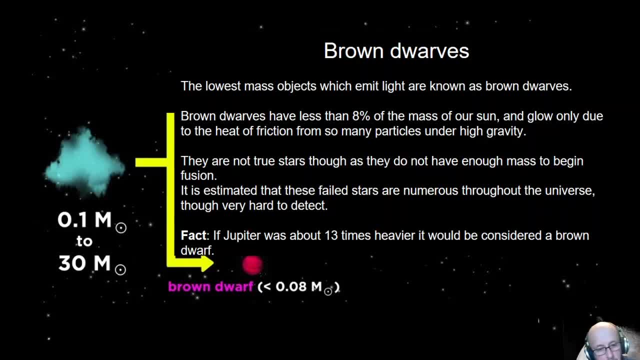 under high gravity. They are not true stars, though, as they do emit some radiation, light, heat, etc. There are estimated that there are numerous of these, but they're very hard to detect. A fact is that Jupiter, which is 13 times heavier than would be considered a brown dwarf could be. 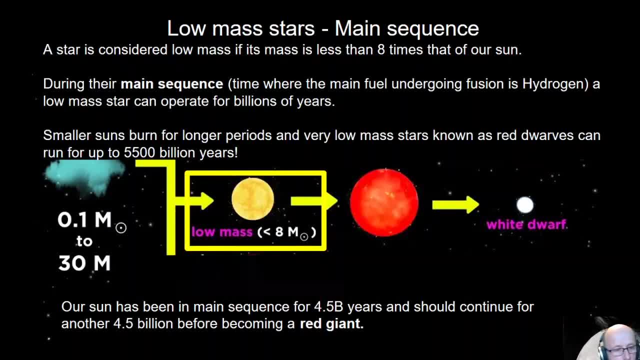 could be the size of a brown dwarf. Now, low mass stars which are in the main sequence and a middle mass are considered brown dwarfs, are basically middle size, are basically low to middle and they're about eight times that of our Sun. is about where we draw the line for this now, basically during the main sequence. 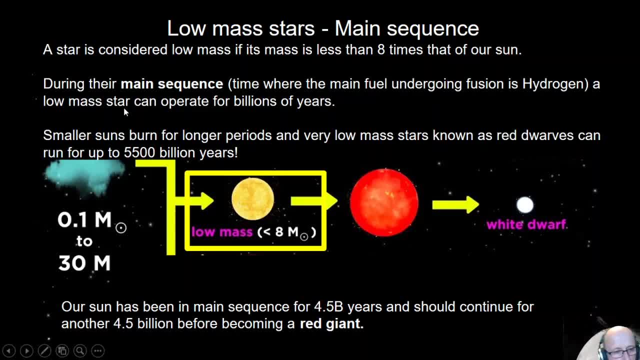 they are fusing hydrogen to form helium and they can now operate for like this for billions of years. for example, our Sun is about mid way through its life cycle and at the moment it is 4.5 billion years old. it's got 4.5 billion years approximately to go. now what is actually? 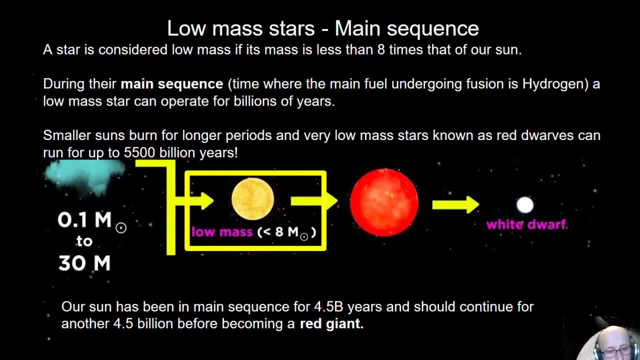 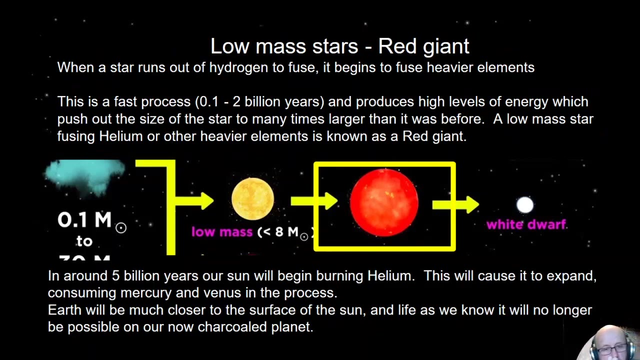 happening is the hydrogen is fusing to helium, so a larger element, but these small Suns can basically burn for long periods and eventually what actually happens is they become red dwarfs and white dwarfs. so first off, they become red giants when the star runs out of hydrogen to fuse. 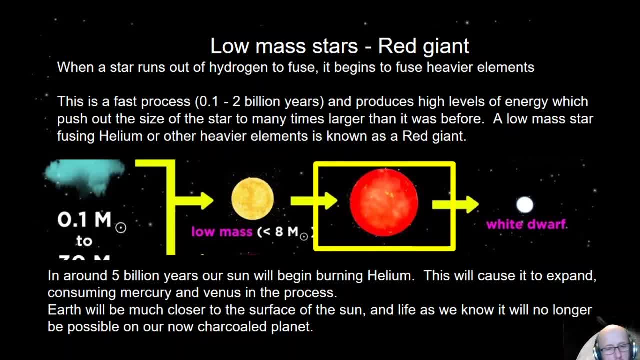 and this is a relatively fast process. it produces high levels of energy which push out from the star and so it becomes much larger. a low mass fusing to helium and then you get larger elements than helium. so you will get lithium and things like that. so in about four and a half to five billion 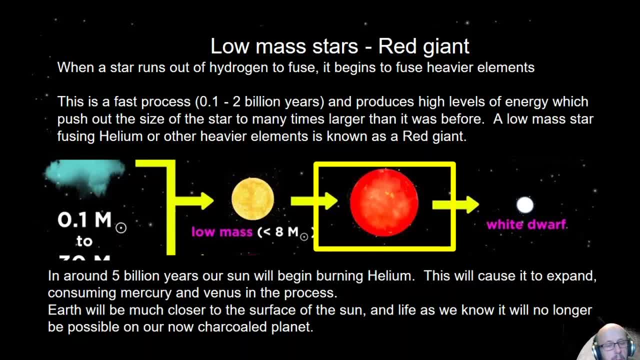 years our Sun will begin running out of hydrogen to fuse and helium to fuse and it will continue or expand consuming hydrogen to fuses. and it will continue to expand, consuming the nearest planets, so Mercury and Venus. Earth will be much closer to the surface of the Sun so we better find another planet before. 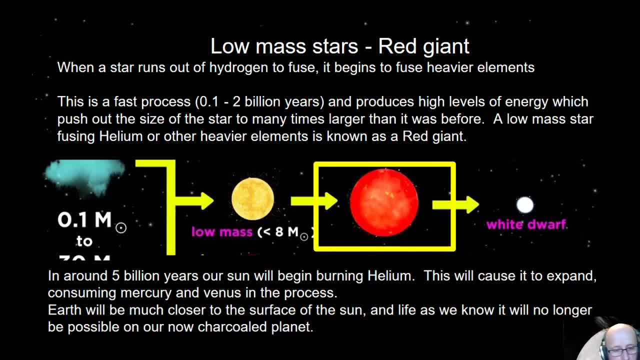 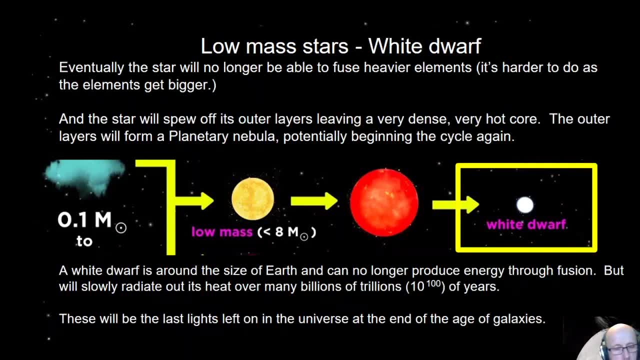 we get there because it will become charcoal. eventually, after the red giant phase, our Sun will go into a white dwarf phase. now low mass stars basically end up in the white dwarf phase and this is where they can fuse elements larger than hydrogen and helium, and you'll find that it can get to elements up to 26, which is 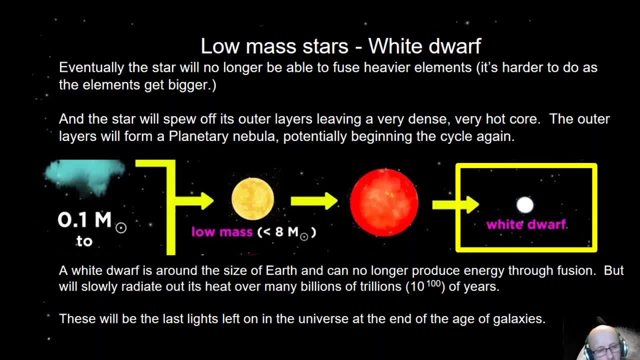 iron on the periodic table. the reason it can do that is because it becomes very dense and it's got a very hot core, okay. so things like iron produce energy for a period of time, and when it is about the size of earth, it can no longer producing. 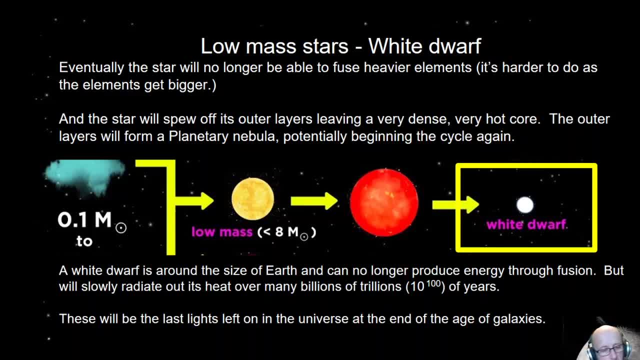 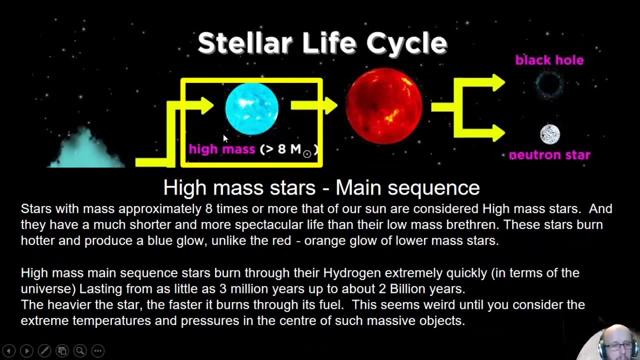 energy via fusion and it will slowly radiate at its heat for billions and trillions of years. now, high mass stars- these are mass of eight times our Sun- can end up in two different pathways. First off, it ends up as a red supergiant and could become a neutron star if it weighs less. 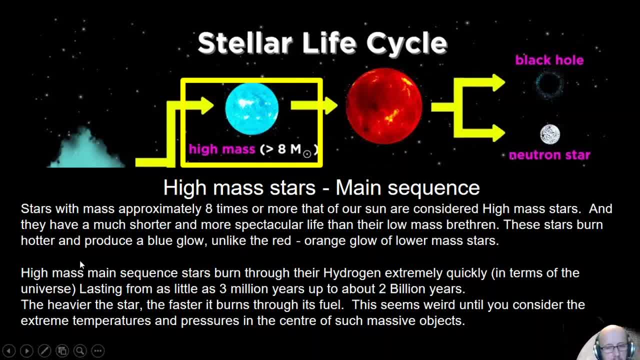 or a black hole. Now, basically, these are very spectacular stars. They have shorter lifespans and they basically fuse and produce a very blue glow, which is higher temperature, and they will continue doing that until gravity impacts on them and they collapse. Basically, high-mass stars will burn through. 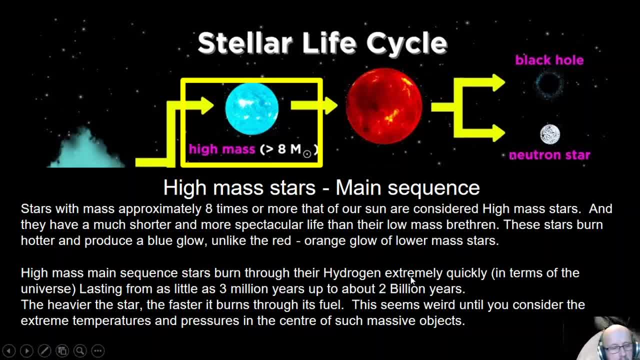 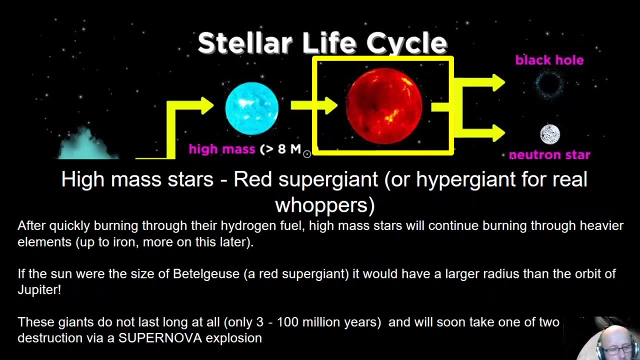 hydrogen extremely quickly and lasting from as little as 3 billion years to 2 billion years, and then when it gets to a certain weight, it gets extreme temperatures and pressures and collapses on itself. So after it produces up to iron, then it can collapse. Now, if the Sun was the size of Betelgeuse, which is the size of the sun, then it would collapse. Now, if the Sun was the size of Betelgeuse, which is the size of Betelgeuse, which is the size of Betelgeuse, which is the size of Betelgeuse, 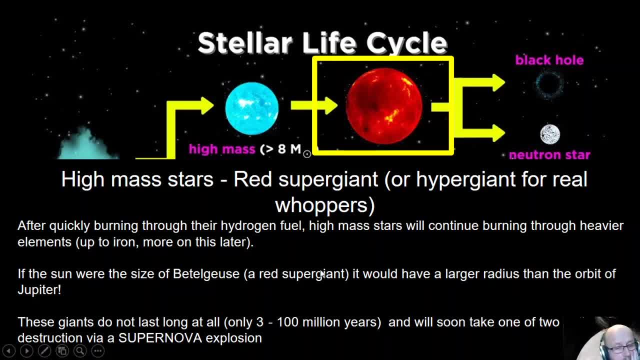 and if it had a red supergiant up near Orion's belt, it would have a radius of about the size of the orbit of Jupiter. so it's enormous. These giant stars do not last long at all and will take one of two pathways via the supernova explosion. 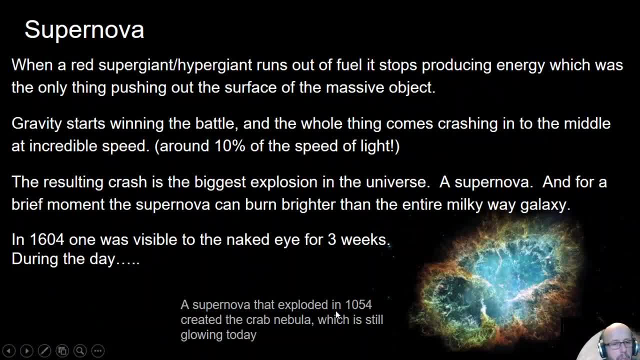 When a red supergiant or hypergiant runs out of fuel, What actually happens is there's a collapse, because gravity is winning the battle. There is not enough fuel for it to be pushed out, So the resulting collapse occurs very quickly and a supernova is formed. 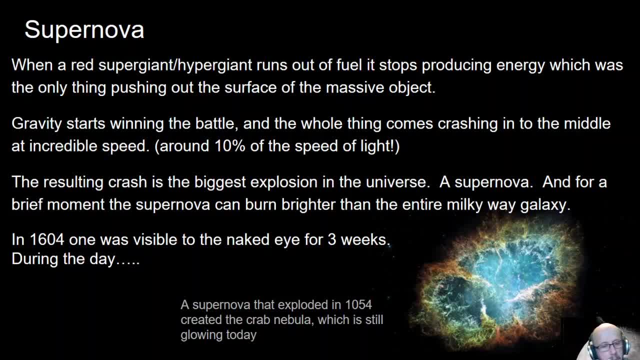 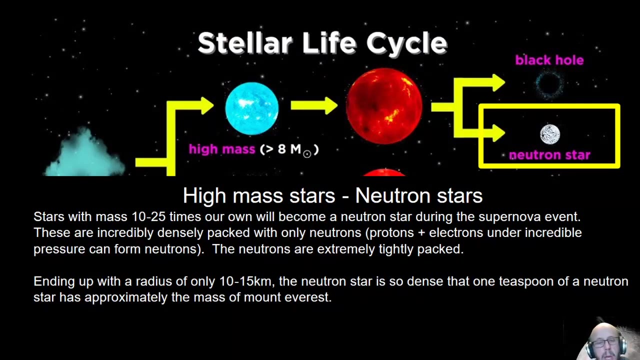 which is the largest explosion in the known universe, And it can burn brighter than the entire Milky Way galaxy. So the supernova that exploded in 1054 created the Crab Nebula, which is glowing today. Stars with about 10 to 25 times our size will become neutron stars. 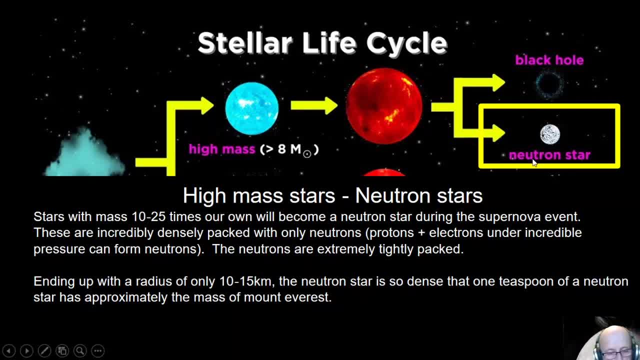 Now these are not as large as black holes and basically the protons and electrons are packed under great pressure and they form neutrons and they're extremely tightly packed. Now neutron stars are very dense with about a teaspoon of neutron weighing the entire mass of Mount Everest. 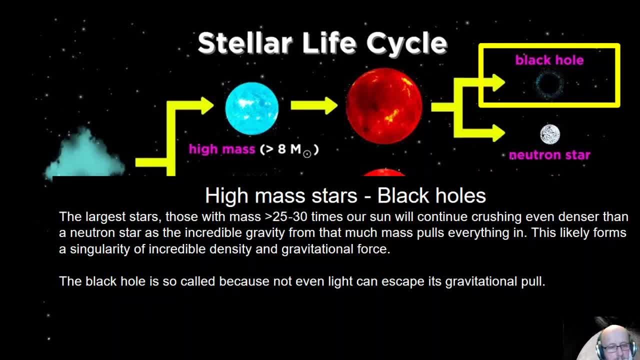 If a star is larger like 25 times the size of our Sun, it will continue crushing even denser and denser. So the red supergiant stage continues until it collapses, And when it collapses you get incredible density and gravitational force. 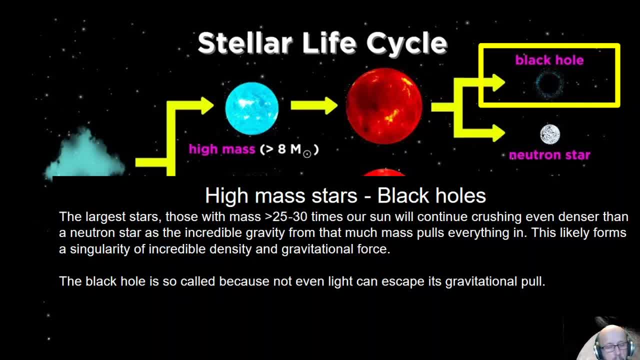 And this is when a black hole is formed. It's called a black hole because not even light can escape its gravitational push. A black hole was pictured a couple of years ago by X-ray detection And it took them a long time to actually form that picture. because of that, 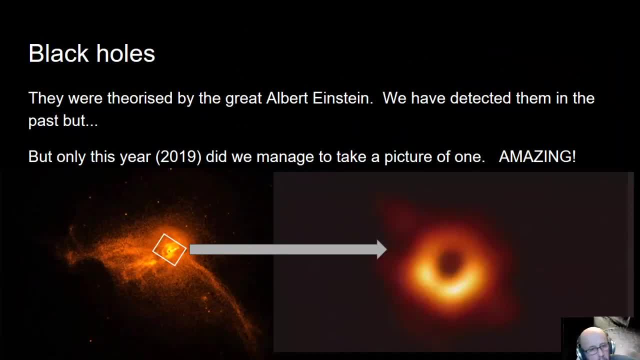 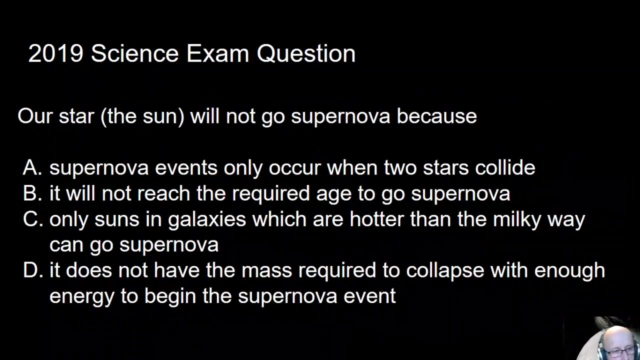 Black holes were actually theorized by Albert Einstein 100 years ago almost, And we have detected them, but we only just in 2019 have been able to take a picture. So this picture was taken via X-ray detection. So a couple of questions for you from the exam.